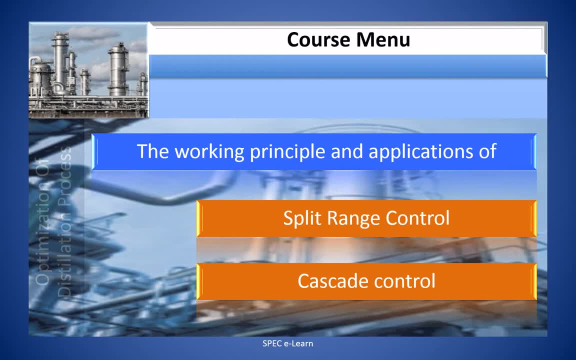 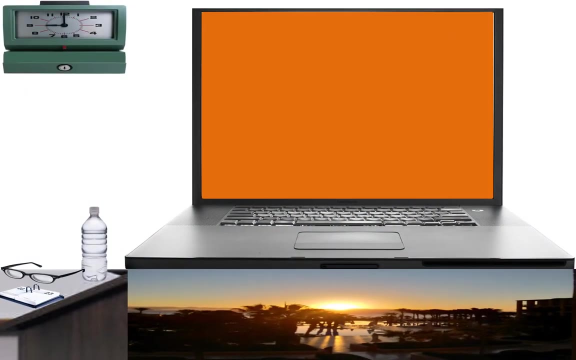 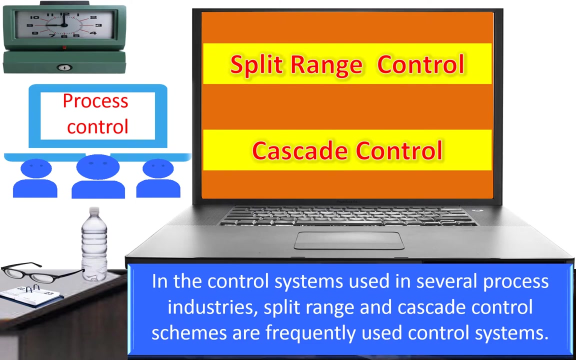 Please subscribe to the channel. By subscribing, you will motivate us to produce more knowledgeable video content for you. So subscribe now, before you forget. In the control systems used in several process industries, Split Range and Cascade Control Schemes are frequently used control systems. 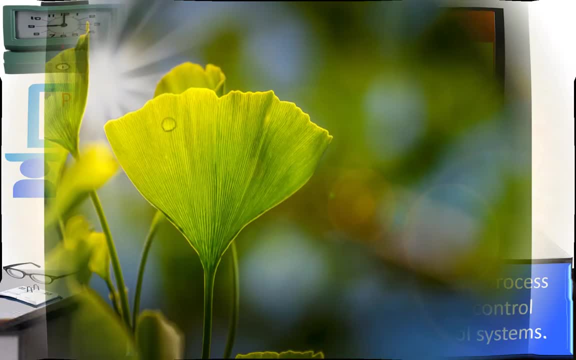 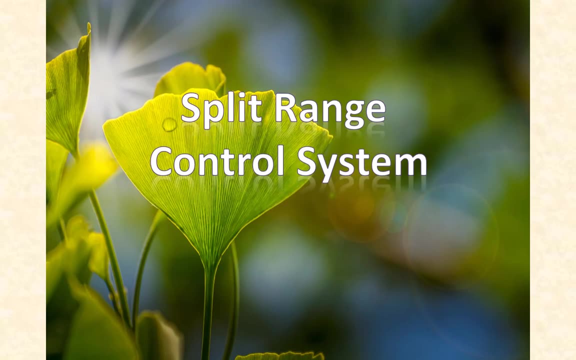 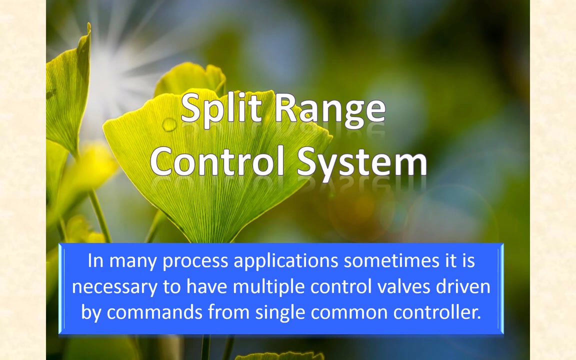 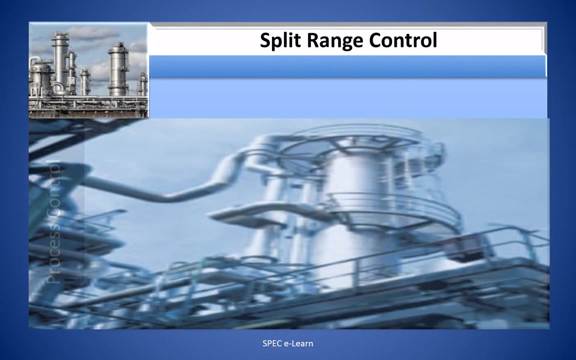 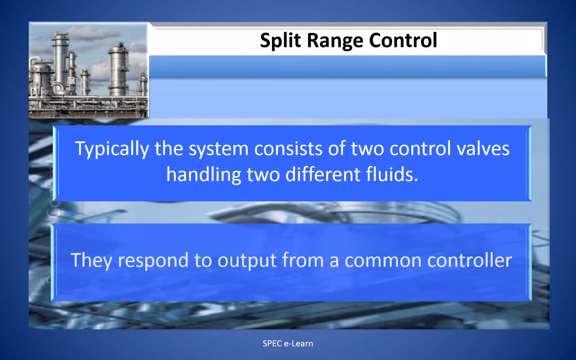 We will discuss these control systems one by one. First, Split Range Control System. First Split Range Control System: In many process applications sometimes it is necessary to have multiple control valves driven by commands from a single common controller. Typically, the system consists of two control valves handling two different fluids. 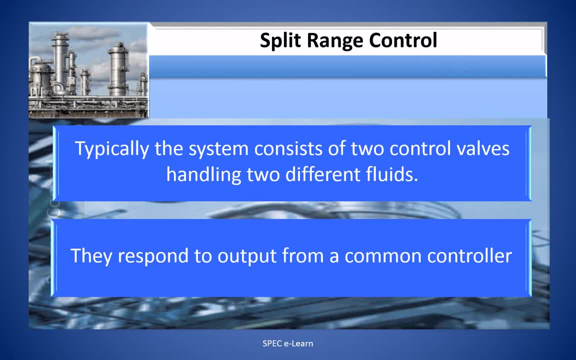 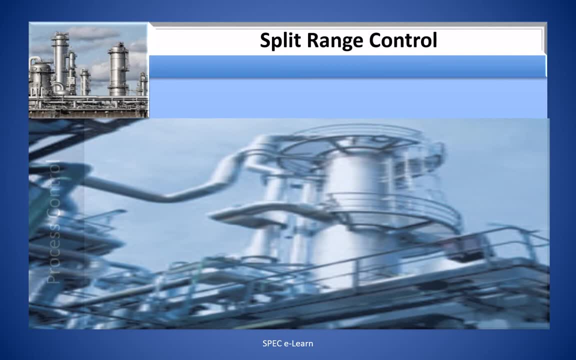 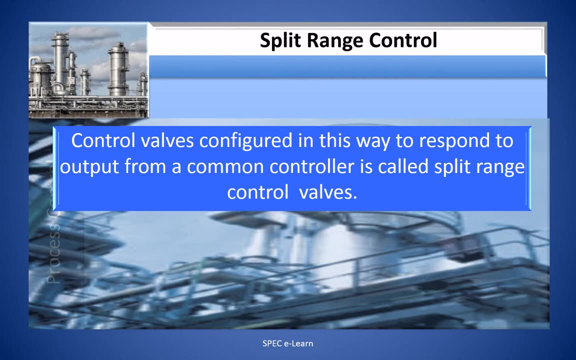 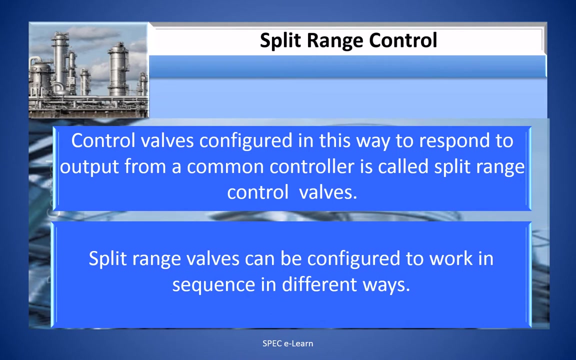 They respond to output from a common controller. They are often speeded by a single controller or by using the control system. Controlled valves configured in this way to respond to output from a common controller is called Split Range Control Valves. Split Range Control Valves can be configured to work in sequence in different ways. 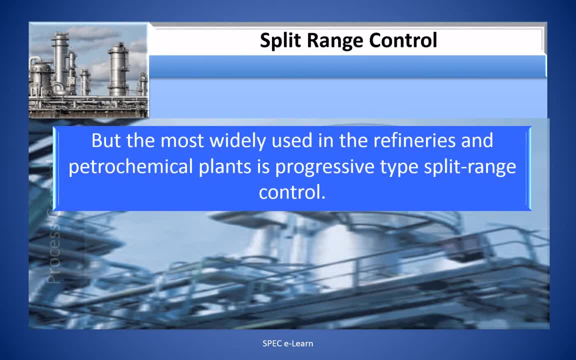 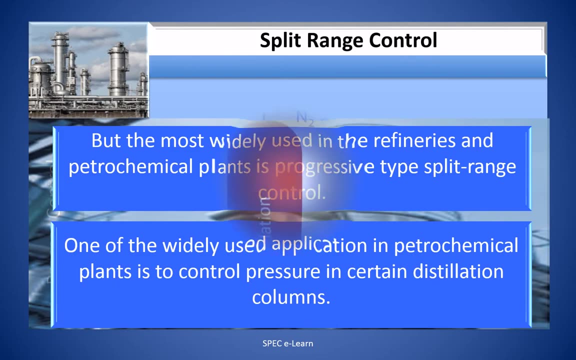 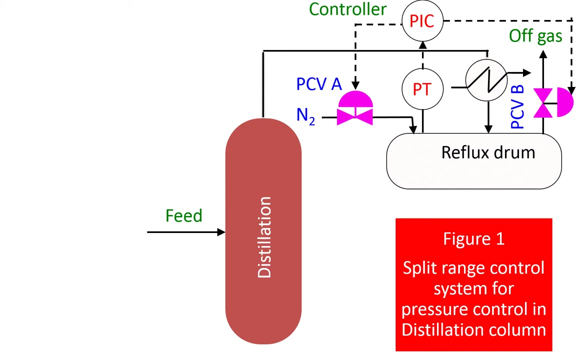 But the most widely used in the refineries and petrochemical plants is progressive-type speed-range control. One of the widely used applications in petrochemical plants is to control pressure in certain distillation columns. The working principle of a speed-range control scheme in a distillation column is illustrated. 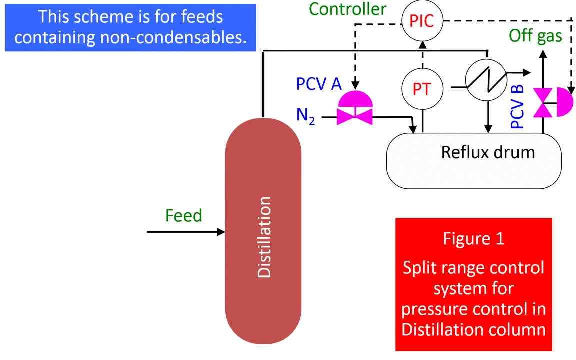 in this figure. In many instances the feed to distillation column consists of light gases which are essentially non-contensibles at the operating pressure and temperature of the column. Hence they accumulate in the reflux drum. Usually, in a distillation column without light gases, cooling water is used to control. 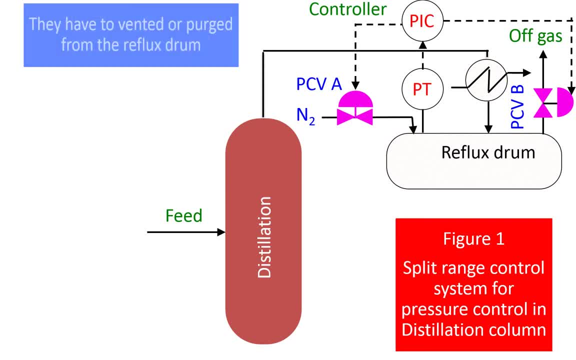 the pressure In columns with feed containing inerts and non-contensibles. the cooling water flows is not the desired method. Instead, the speed-range control method is used. Two pressure control valves: one, a nitrogen valve that outputs nitrogen into the reflux drum, and another pressure control valve that lets the non-contensibles to go. 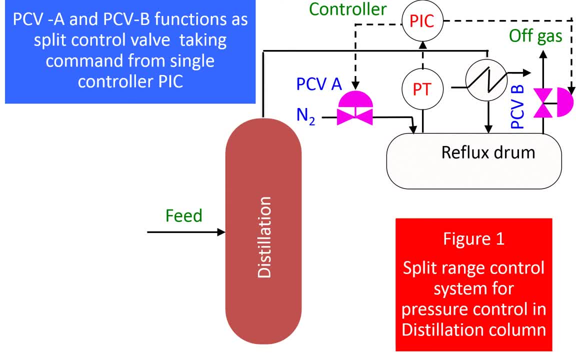 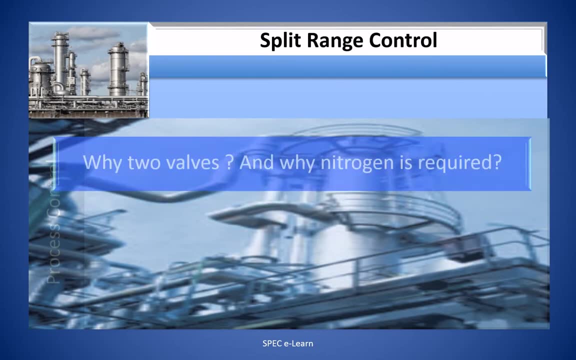 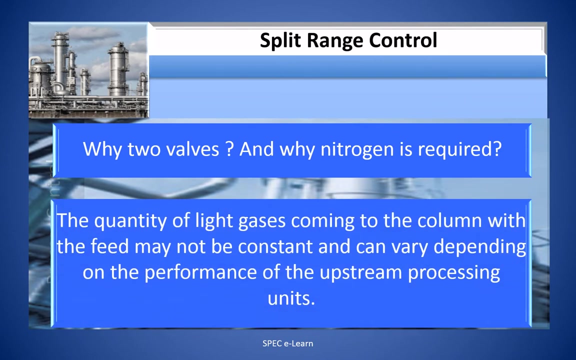 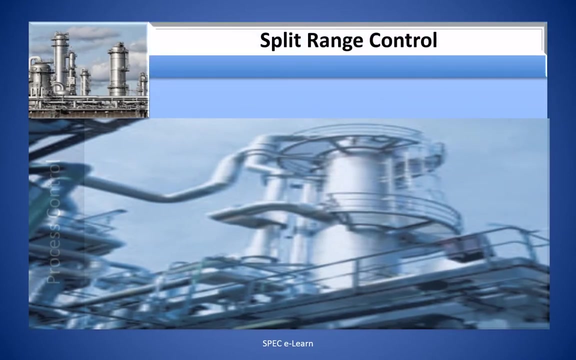 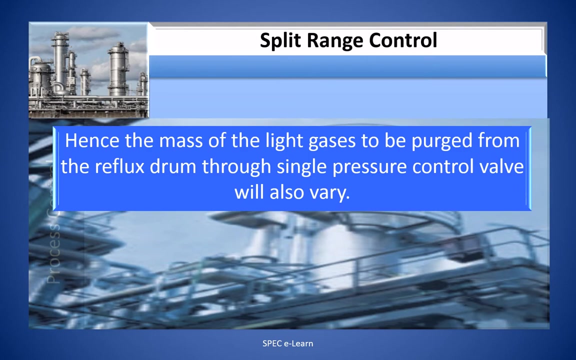 to the atmosphere by purging. Why two control valves And why nitrogen is required? The quantity of light gases coming into the column along with the feed may not be constant and can vary depending on the performance of the upstream processing units. Hence the mass of the light gases to be purged from the reflux drum through a single pressure. 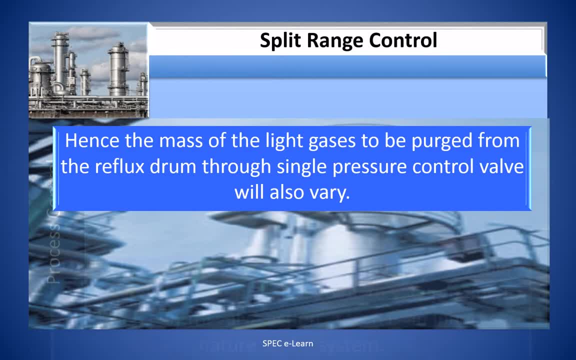 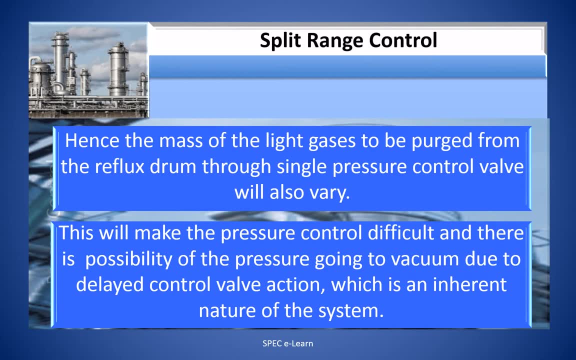 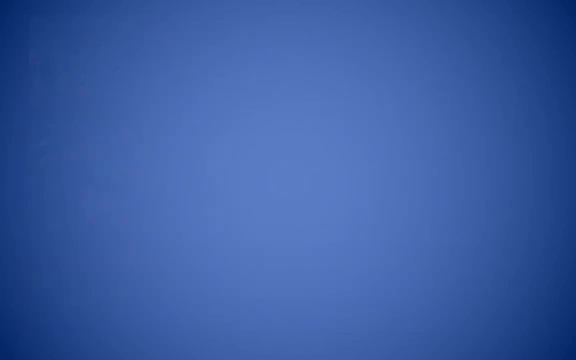 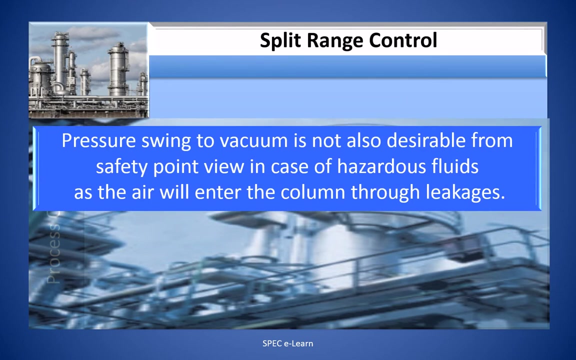 control valve will also vary. This will make the pressure control difficult and there is a possibility of the pressure going into vacuum due to delayed control valve action, which is an inherent nature of the system. Pressure swing to vacuum is not also desirable from safety point of view in case of hazardous 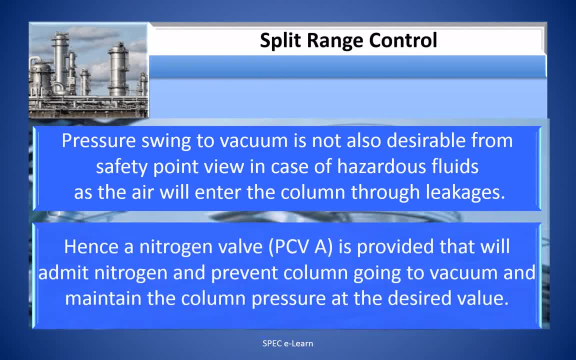 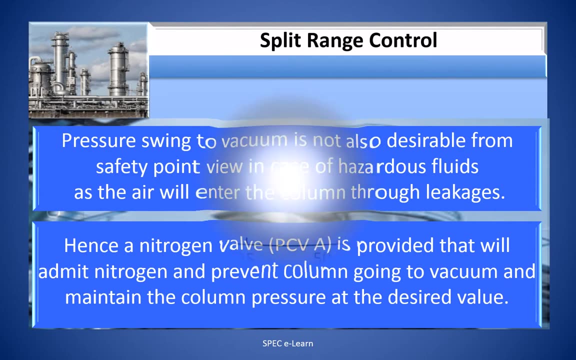 fluids as air will enter the column through the leakages. Hence nitrogen valve- PCVA- is provided that will admit nitrogen and prevent column going to vacuum and maintain the column pressure at the desired value. This figure illustrates the function of a split-range control valve. 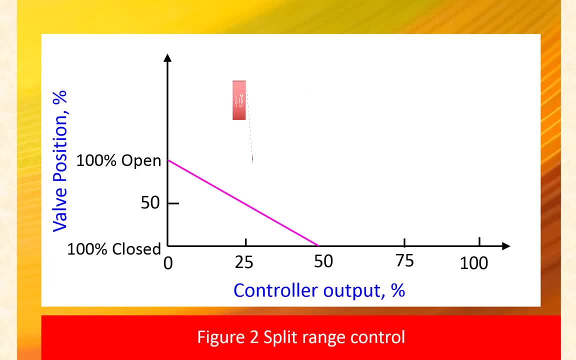 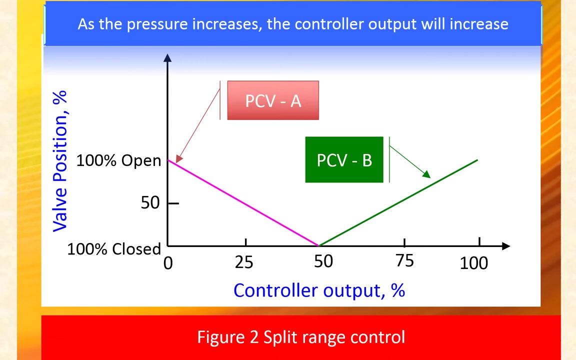 valve with valve opening versus pressure controller output diagram. Initially the control valve PCVA is fully open and PCVB is fully closed. At this point the pressure increases above the set point, The controller output starts increasing from zero and the control valve PCVA begins to close At 25%. 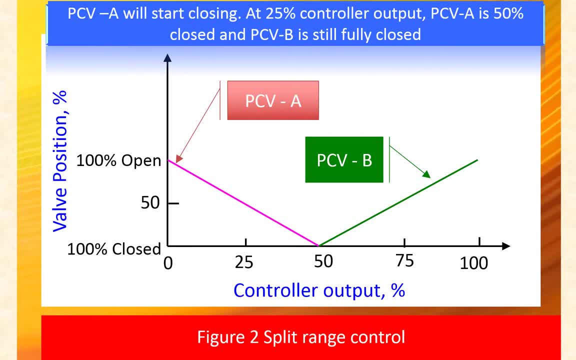 output of the controller, the PCVA is 50% closed and the control valve PCVB is still fully closed. As a controller output increases to 50%, the control valve PCVA goes to full close and PCVB still remains fully closed. you. 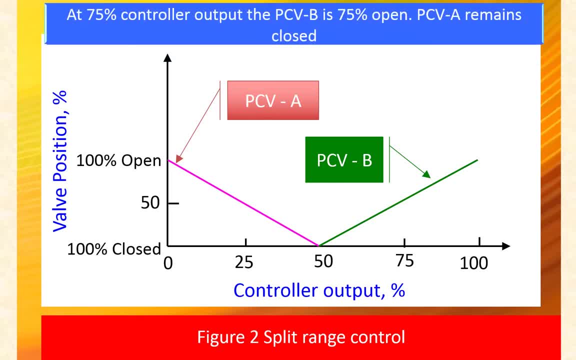 As the output increases beyond 50%, the PCVB starts opening. At control output of 75%, PCVB is 50% open. As the control output increases to 100%, the PCBV goes to full open and PCVA still remains closed. 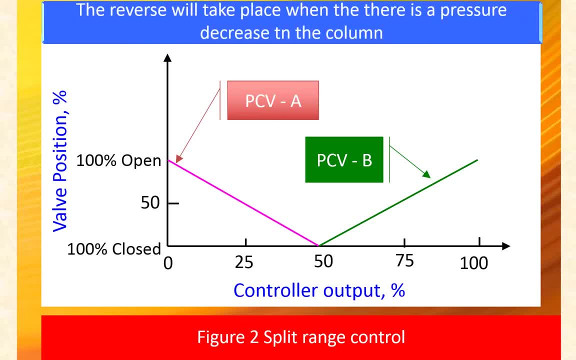 The reverse will take place. when there is a pressure decrease in the column, The PCVB will close first. When it is closed, if the pressure continues to decrease, the controller output will decrease below 50% and the second valve, PCVA, will begin to open and allow the nitrogen to come in to maintain the pressure. 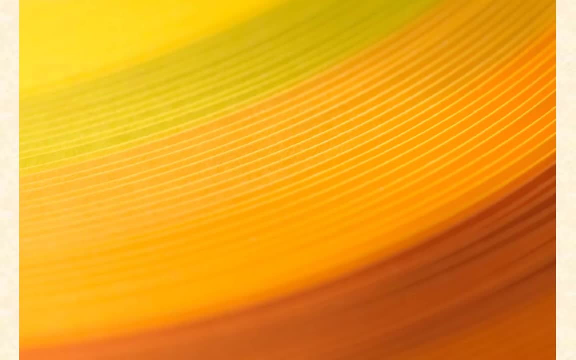 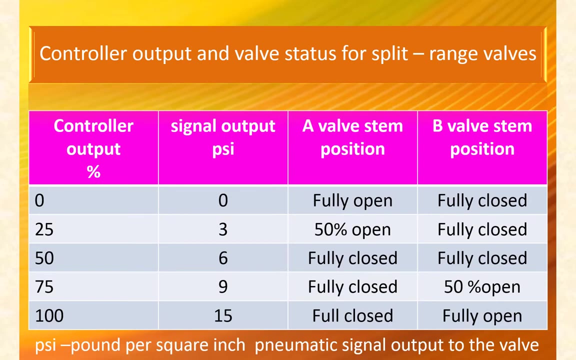 This table represents the controller output to the two split-range control valves and their response and position. Control output: 0%. corresponding signal output in PSI 0.. A valve position: full open. B valve position: full- close. Control output: 25%. Signal output: 3 PSI. A valve position: 50% open. B valve position: full close. 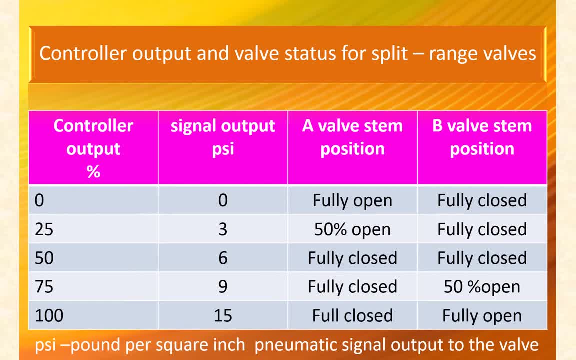 Control output: 50% Signal output: PSI: 6 PSI A valve position: full close. B valve position: full close At 50% output. both A and B are fully closed. Control output: 75% Signal output: 9 PSI A valve position: full closed. 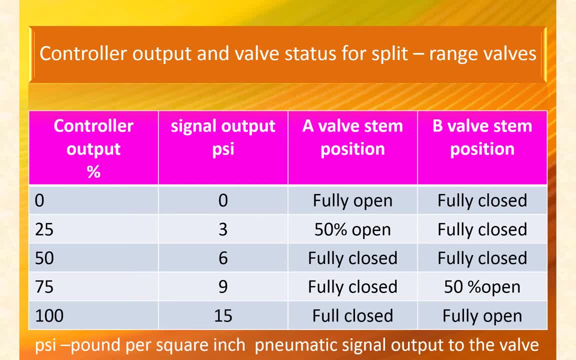 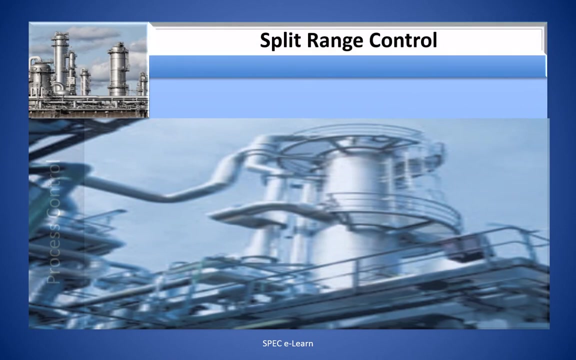 CYB is fully closed. B valve position: 50% open. Control output: 100% Signal output: 15 PSI. A valve position: full closed. B valve position: fully open: CYB 13.. CYB 13 is fully closed. Another application of swell current control is in the application of. 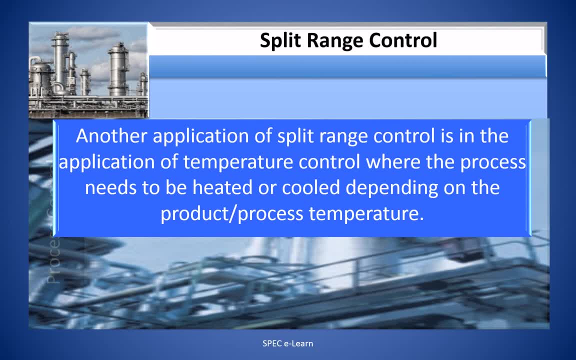 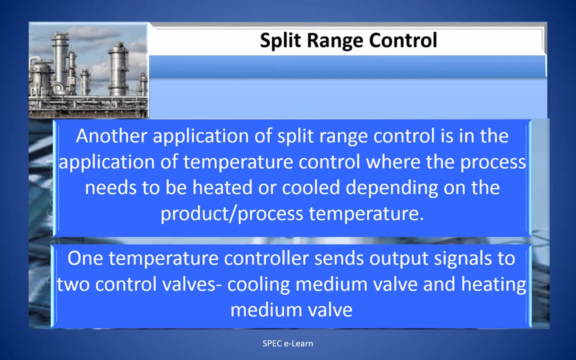 control internal determinants, 말씀 is in the application of temperature control where the process needs to be heated or cooled, depending on the product or process temperature. One temperature controller sends output signals to two control valves: cooling medium valve and heating medium valve. 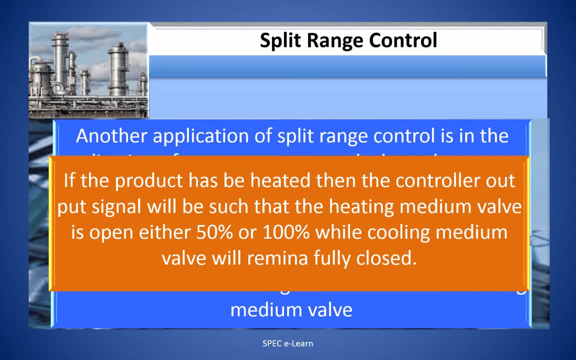 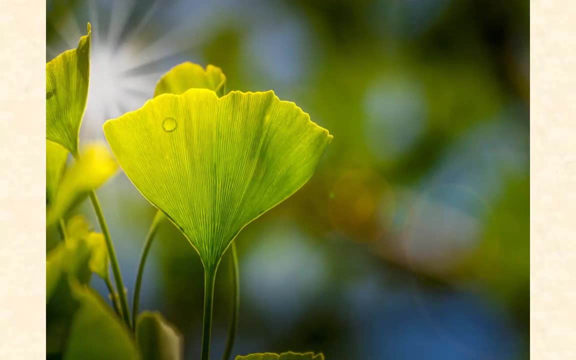 If the product has to be heated, then the controlled output signal will be such that the heating medium valve is open either 50% or 100%, but the cooling medium will remain fully closed. Having discussed split range control system, we will move on to cascade control system. 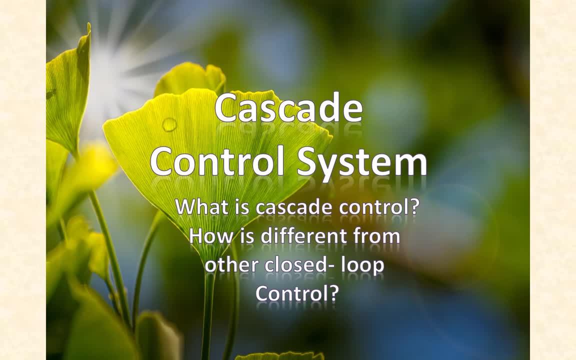 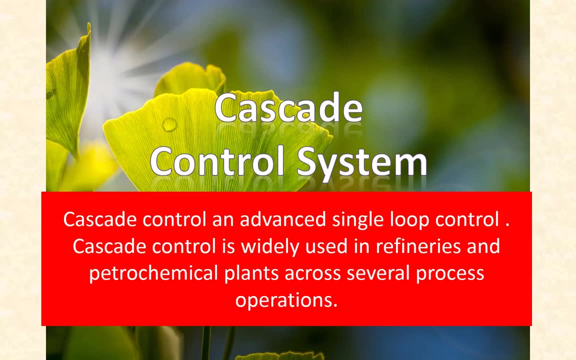 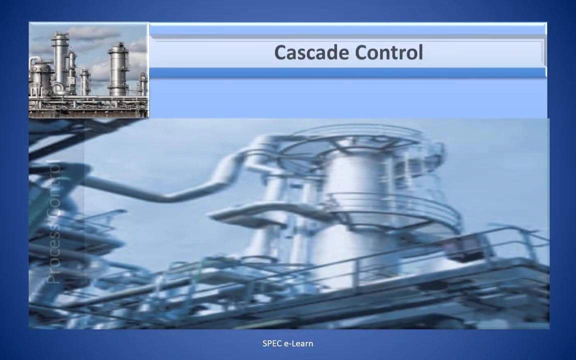 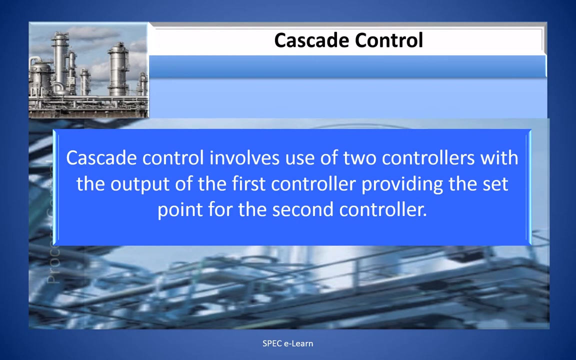 What is cascade control? How is it different from other closed loop control? Casual control is an advanced single loop control. Cascade control is widely used in refineries and petrochemical plants across several process operations. Cascade control involves use of two controllers, with the output of the first controller providing 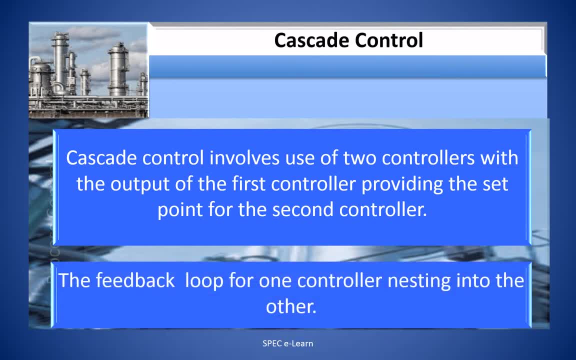 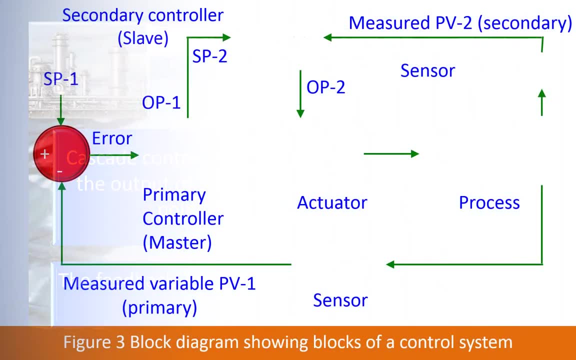 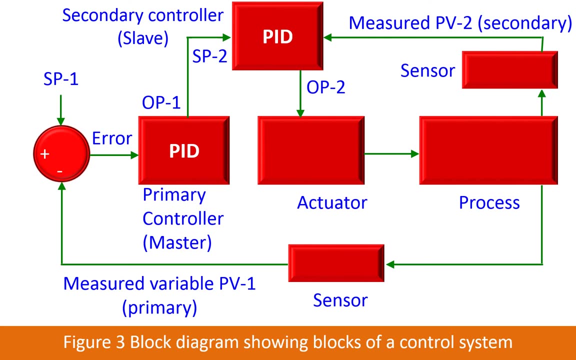 the set point for the second controller, The feedback loop For one controller nesting into the other. The cascade control concept is illustrated in this block diagram. There are two controllers: a primary controller and a secondary controller. The output of the first or the primary controller, QP1, is used as the set point. SP2 of the secondary. 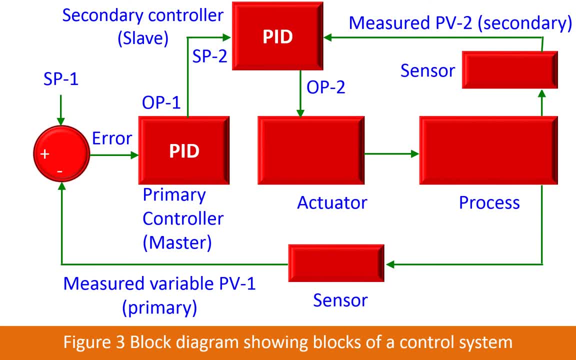 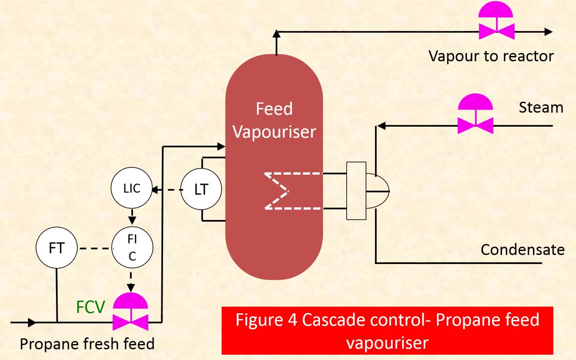 controller. The primary controller is called the master and the secondary controller is called the slave. The slave follows the master. To make your understanding of the concept better, let me give an illustration of a rare world example. in a petrochemical plant, Shown in the sketch is a propane vaporizer. 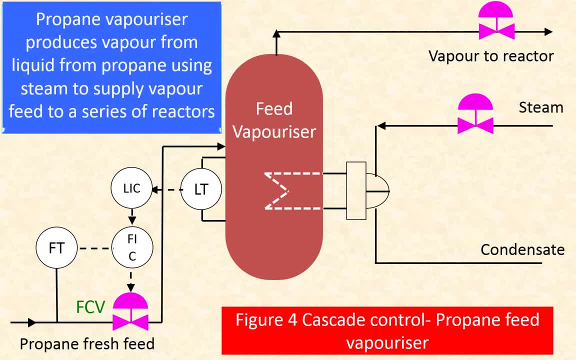 This is a propane vaporizer. It produces vapor from liquid propane. This is a propane vaporizer. This is a propane vaporizer. This is a propane vaporizer. The vaporizer is saponified and is used to supply vapor. The vapor is then filled with a series of reactants using steam to supply a vapor feed. 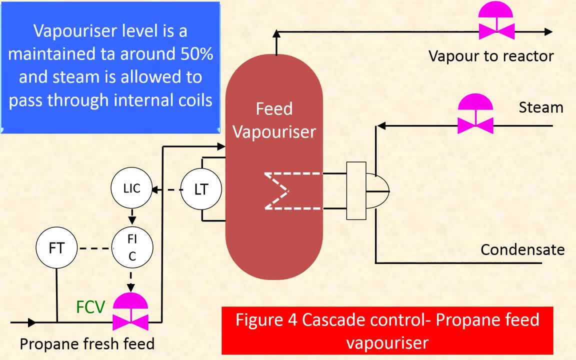 to a series of reactors. Vaporizer level is maintained at around 50% and steam is allowed to pass through the internal coils. The feed to the vaporizer is monitored with a flow meter and regulated by a flow control valve. The whole scheme works on cascade control concept. 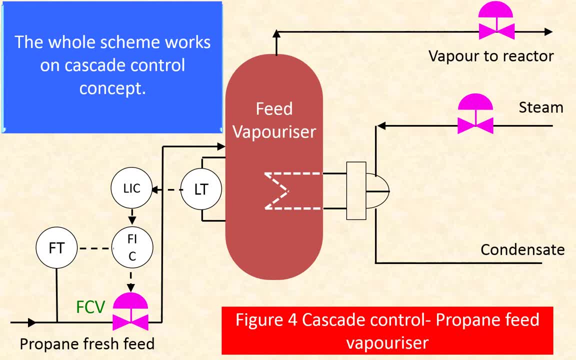 The level in the vaporizer is measured by a level measuring instrument. The same is applied to the second controller. The rate of vaporization is calculated by the state of the vapor. The level is calculated by the state of the vapor and the transmitter signal PV1, is sent to the level controller LIC The output. 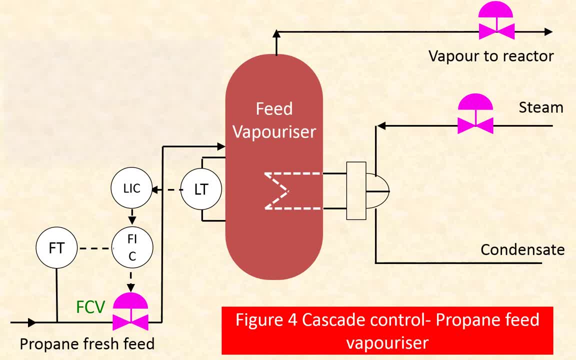 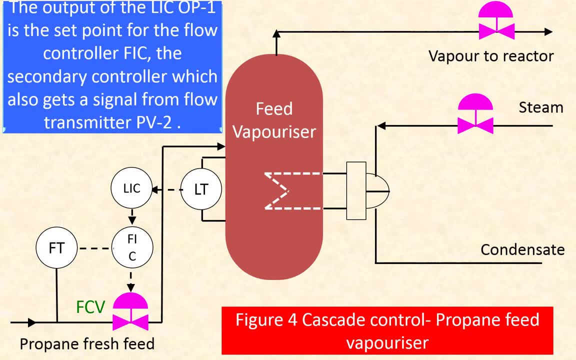 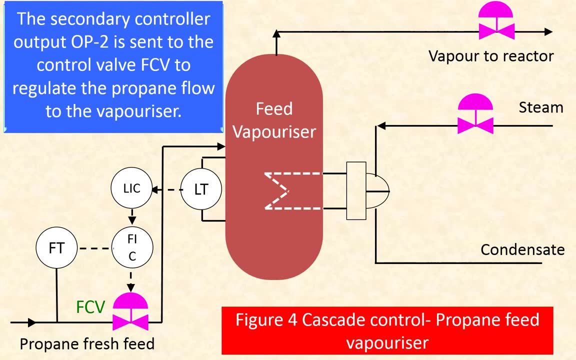 of the LIC. OP1 is a set point to the flow controller FIC, the secondary controller which also gets a signal from the flow transmitter PV2.. The secondary controller output OP2 is sent to the control wall FCV to regulate the propane flow to the vaporizer. The LIC is a master and FIC is a slave. 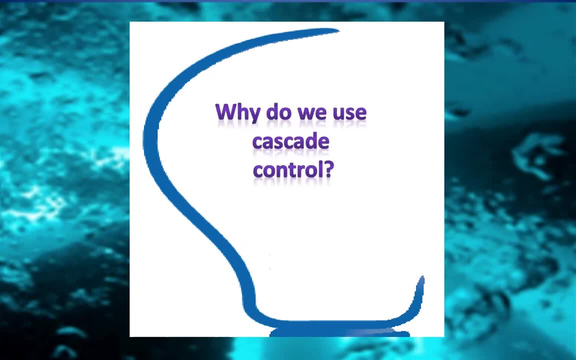 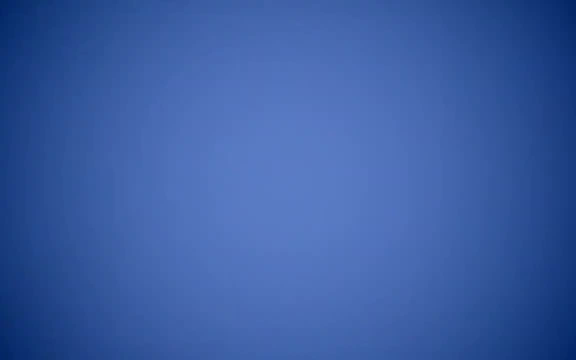 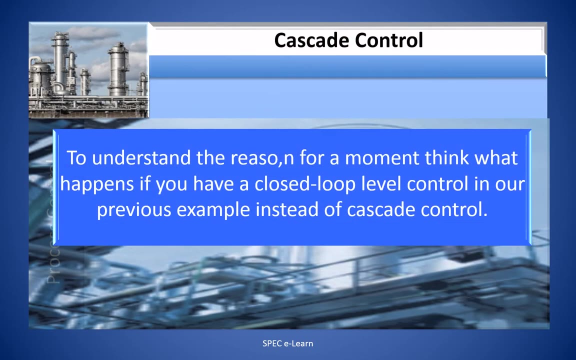 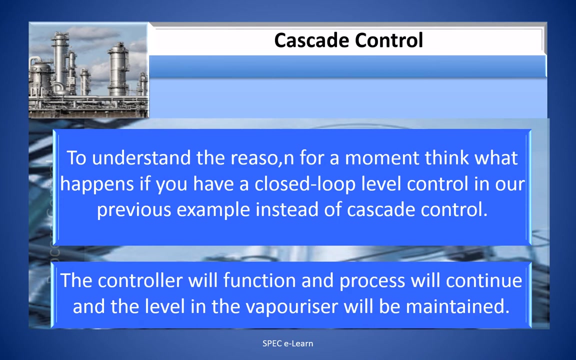 Why do we use cascade control? What are the advantages and disadvantages? To understand the reason, for a moment, think what happens if you have a closed-loop control in our previous example instead of cascade control. The control will function and process will continue and the level in the vaporizer will be maintained. 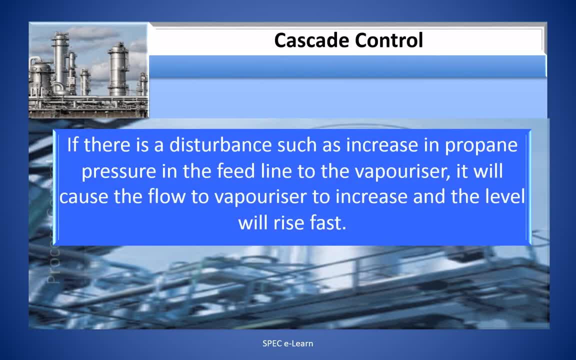 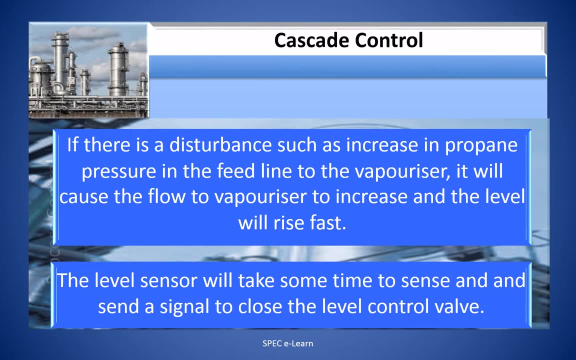 If there is a disturbance, such as an increase in propane pressure in the feed line to the vaporizer, it will cause the flow to vaporizer to increase and the level will raise fast. The level sensor will take some time to sense and send a signal to close a level control valve. 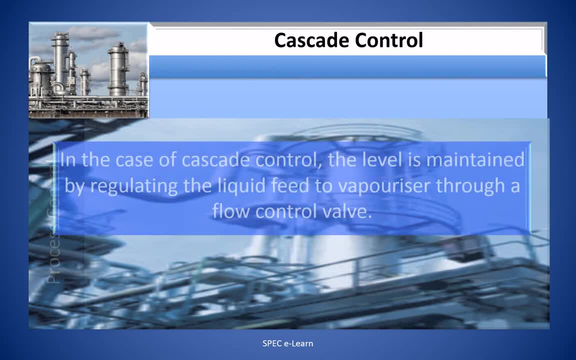 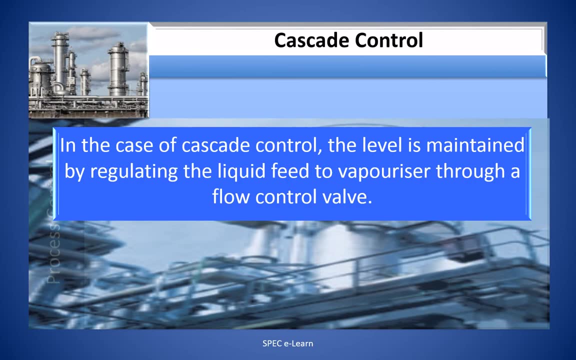 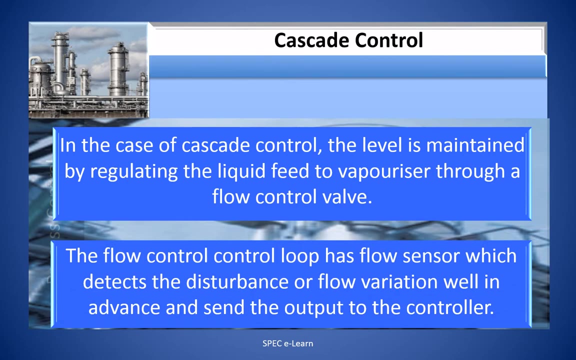 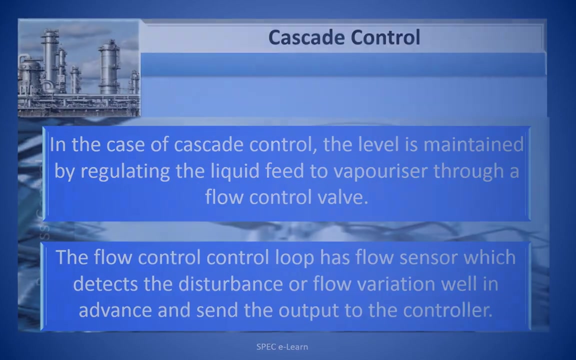 In the case of cascade control, the level is maintained by regulating the liquid flow to the vaporizer through a flow control valve. Here the flow control loop has a flow sensor which detects the disturbance or flow variation well in advance and sends the output to the controller. 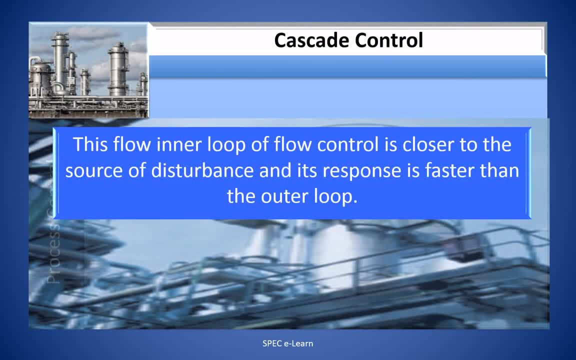 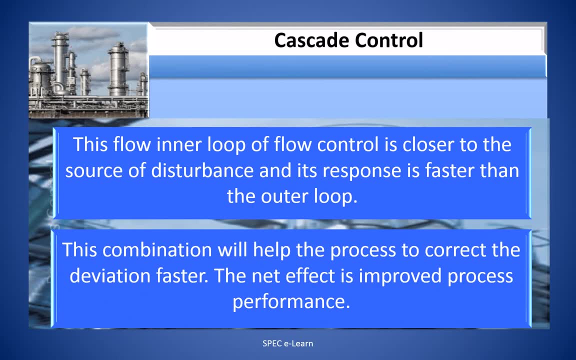 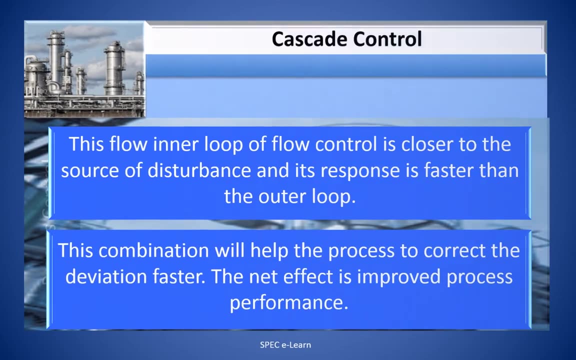 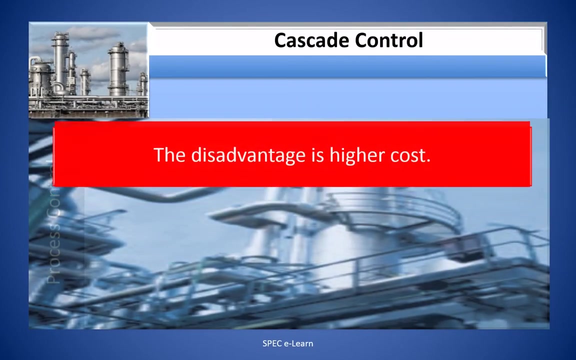 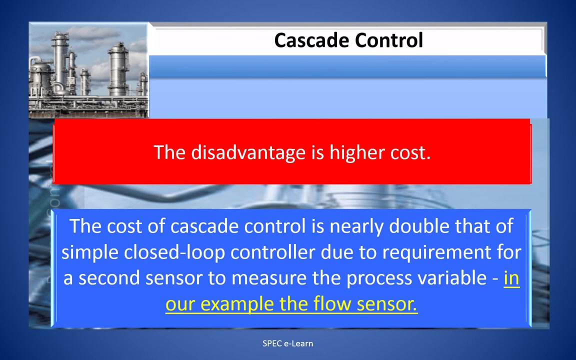 This inner loop of flow control is closer to the source of disturbance and its response is faster than the outer loop. This combination will help the process to correct the deviation faster. The net effect is improved process performance. The disadvantage is higher cost. The cost of cascade control is nearly double that of a simple closed loop controller due 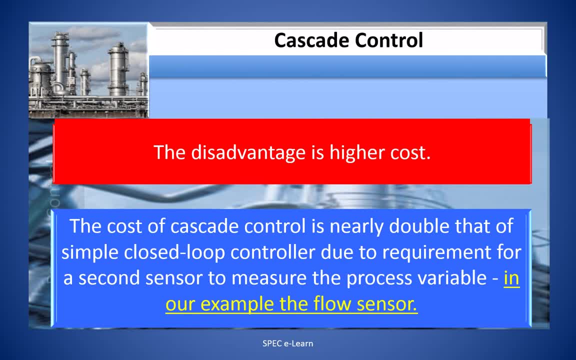 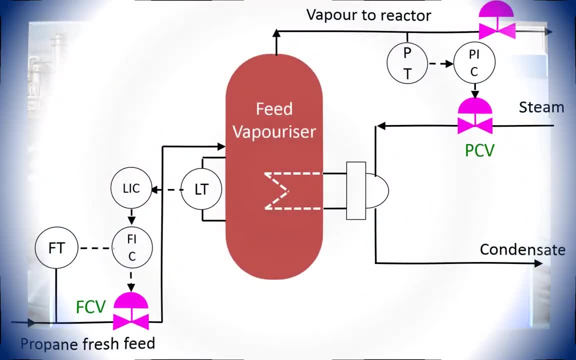 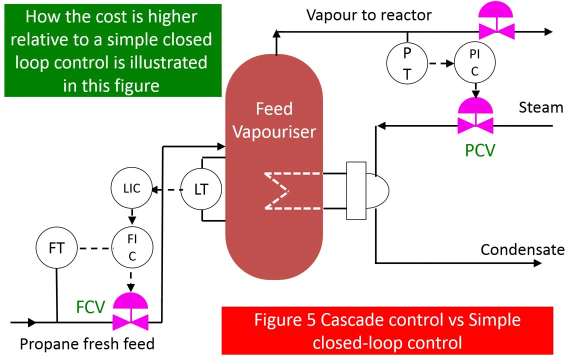 to the requirement for a second sensor to measure the process variable, In our example the flow sensor. How the cost is higher relative to a simple closed loop control is illustrated in this figure. The vaporizer pressure control is a simple closed loop control. 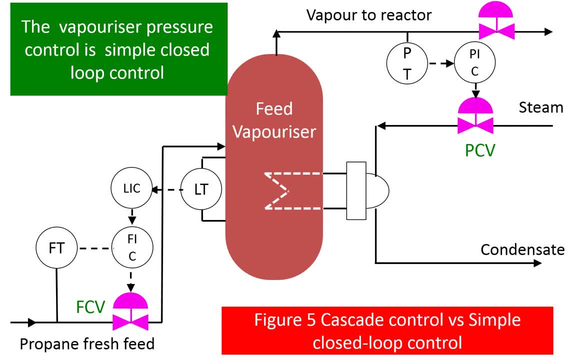 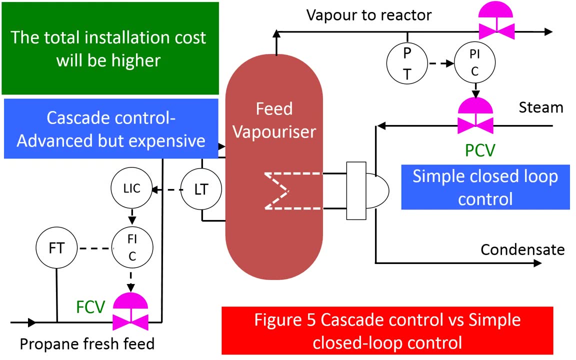 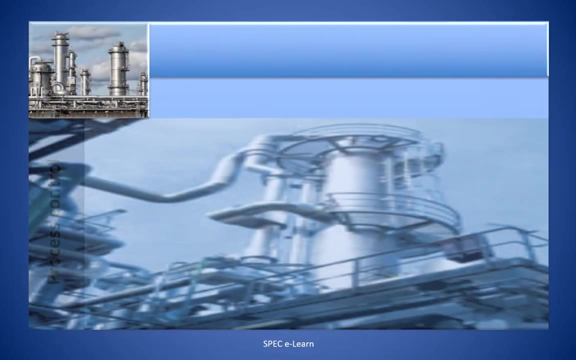 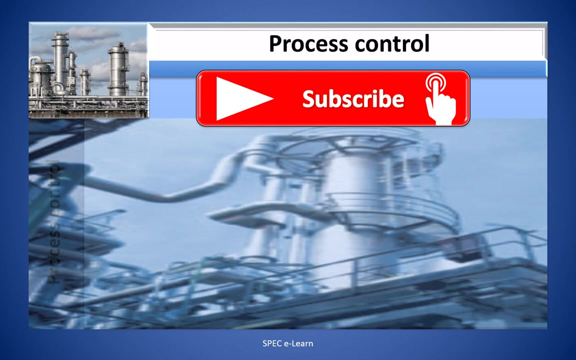 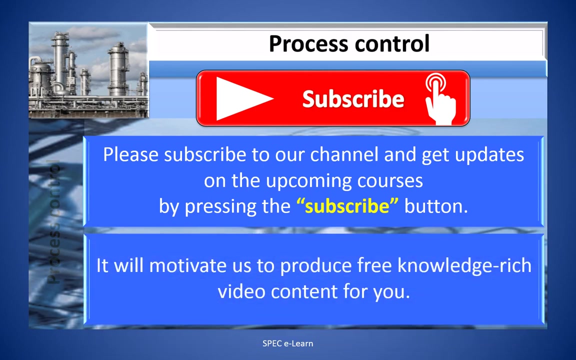 The level control is a cascade control. The cascade control has additional sensors, associated instrumentation network. Hence the total installation cost will be higher. Please subscribe to our channel and get updates on the upcoming courses by pressing the subscribe button. It will motivate us to produce free knowledge. 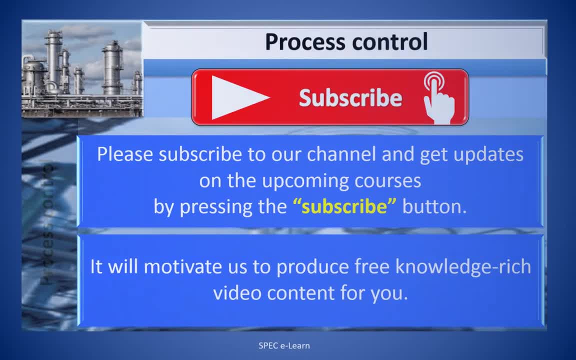 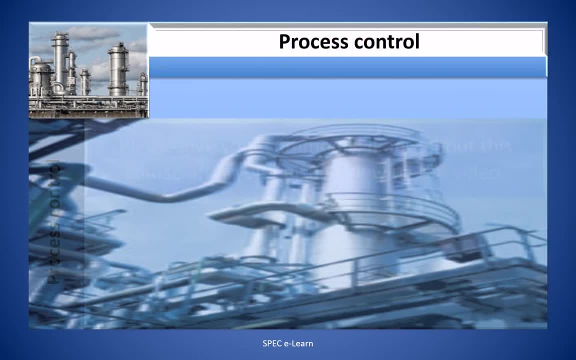 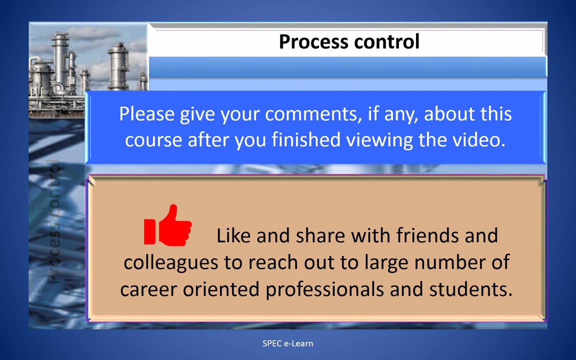 rich video content for you. With this, we have come to the end of the presentation. Please give your comments, if any, about this course after you finished viewing this video. Share with your friends and colleagues to reach out to large number of career oriented professionals to help you. 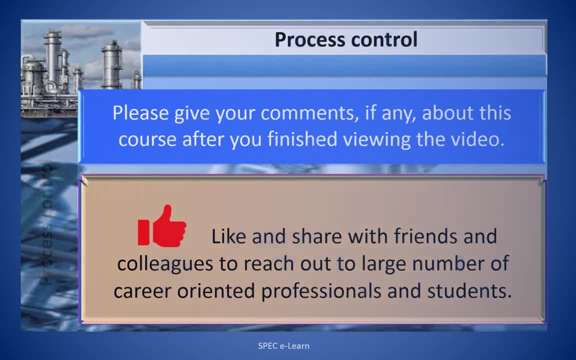 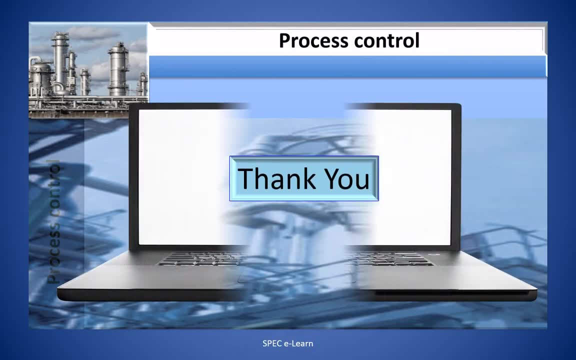 Thank you, students, Thank you for watching. 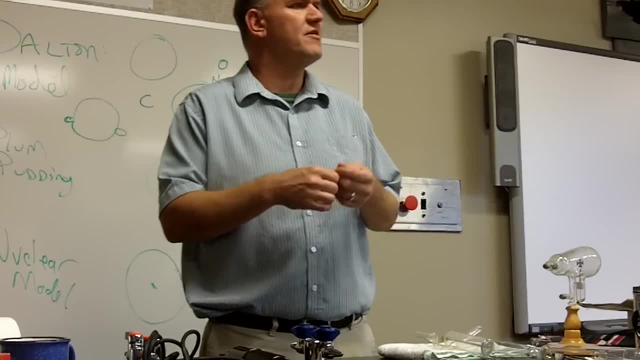 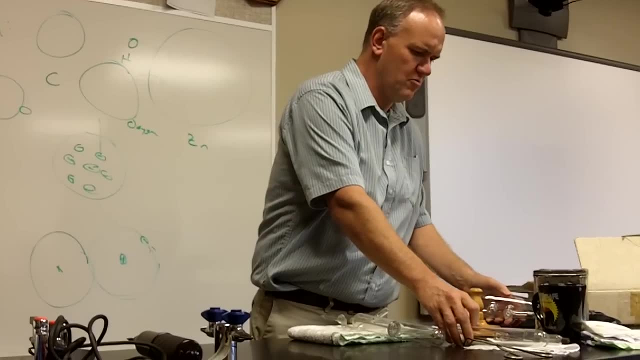 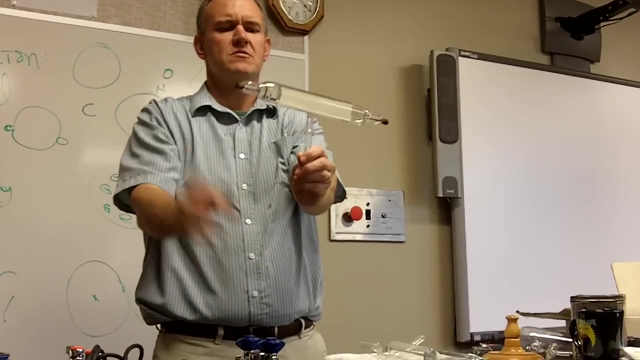 So what I'm going to show you today is how they figured out that Dalton's model was not complete And it began with this thing called a Crookes tube. Has anyone seen a Crookes tube before? This is a Crookes tube. What it is is: it's a tube of glass. that's mostly. 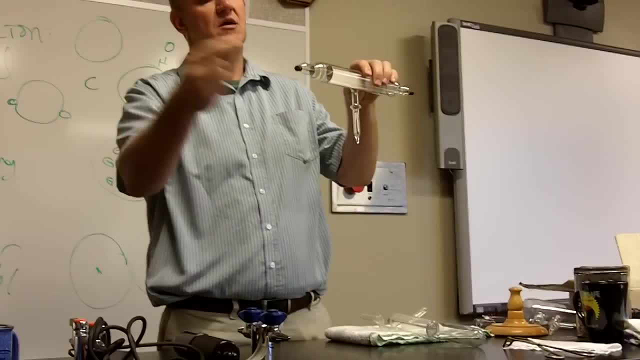 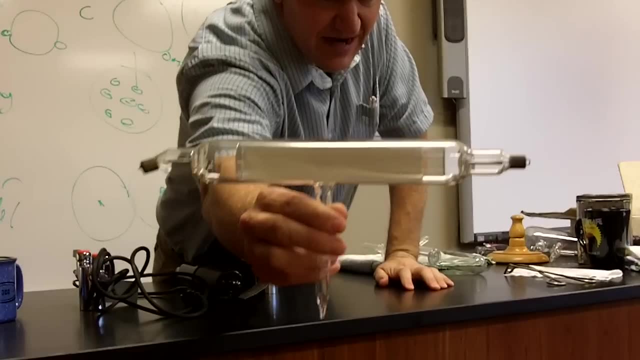 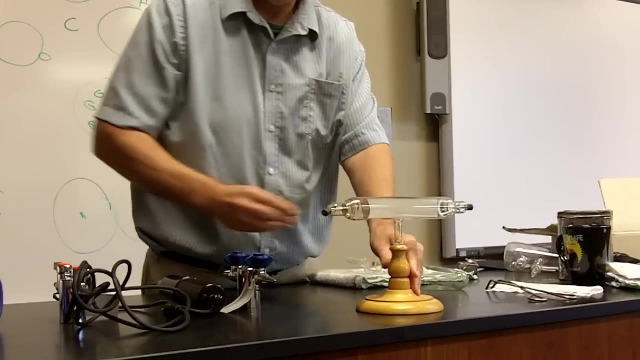 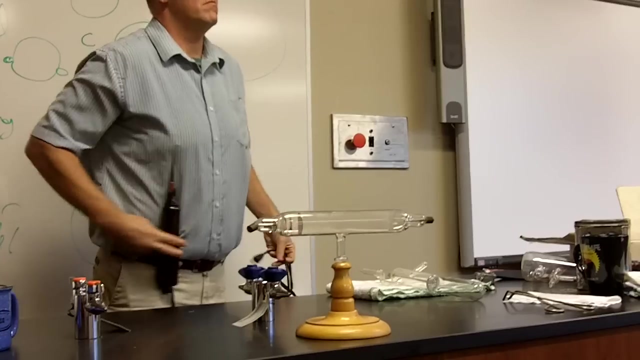 evacuated, meaning most of the air is taken out of it, and it's got an electrode on this side and an electrode on that side. If you look on the inside of it, there's a white screen and the white screen is there for reasons I'll show you in a moment. This is: 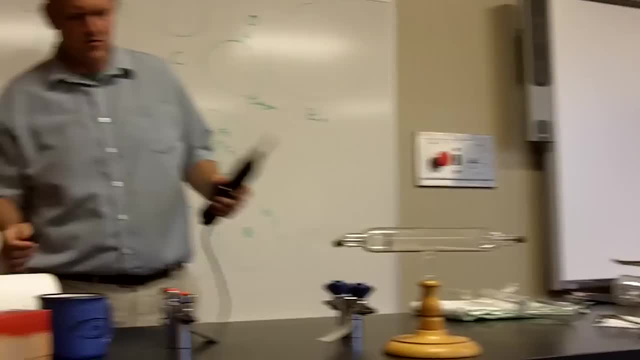 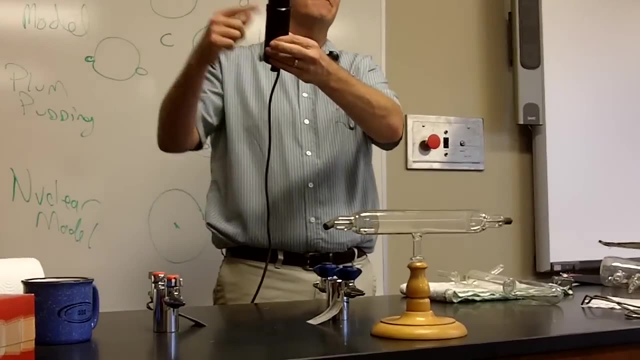 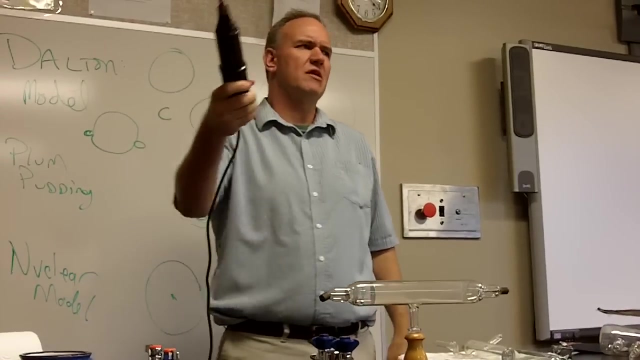 a Tesla coil. Tesla coils generate lots of voltage. So right now there's a magnet on the inside of here that's spinning and it's got some wires around that magnet. It's generating a lot of voltage as it spins because it's a strong magnet. In fact, if I hold another 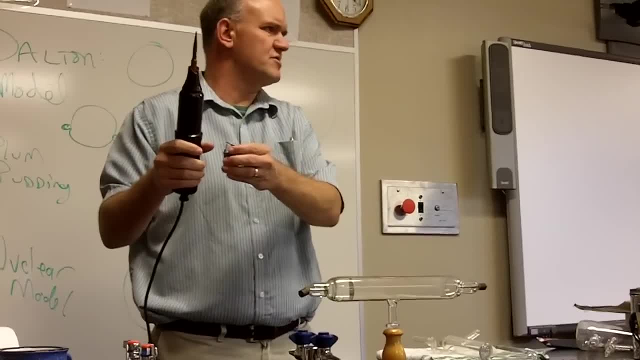 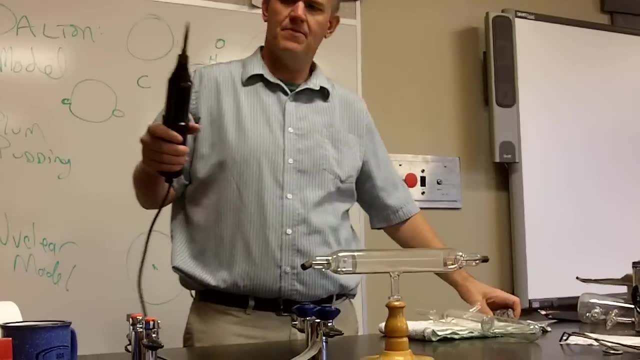 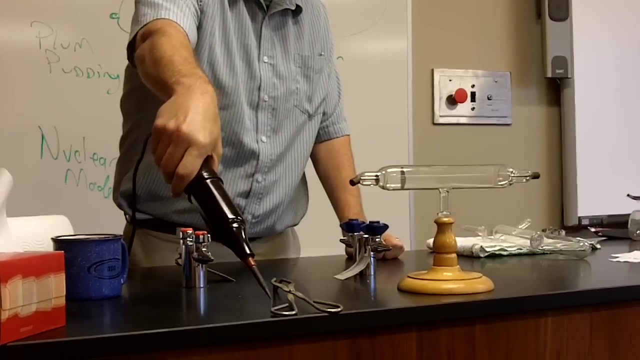 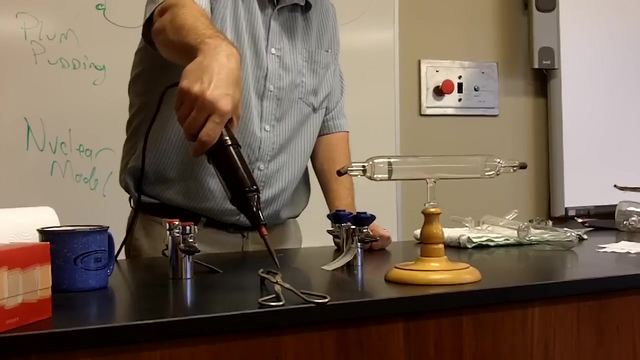 magnet up here. I can feel it vibrating from the spinning of the magnet, Kind of like your rumblers on your game controllers. But this is generating a lot of electricity. You can see that if you hold it up to something metal, People always ask what will happen if you. 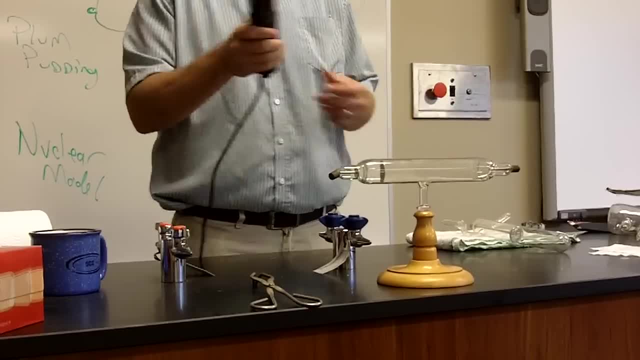 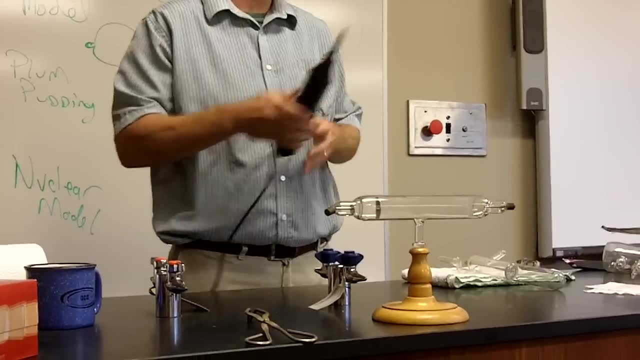 touch it And the answer is: you'll die. That's why I am now dead, A little bit uncomfortable, But in any case, here's what happens when you hold it across a Crookes tube. This is a metal magnet. You can see that if you hold it up to something metal, People always ask. what will happen if you touch it, And the answer is: you'll die. This is a metal magnet. If you hold it up to something metal, People always ask what will happen if you touch it, And the answer is: you'll die. That's why I am now dead A little bit uncomfortable.